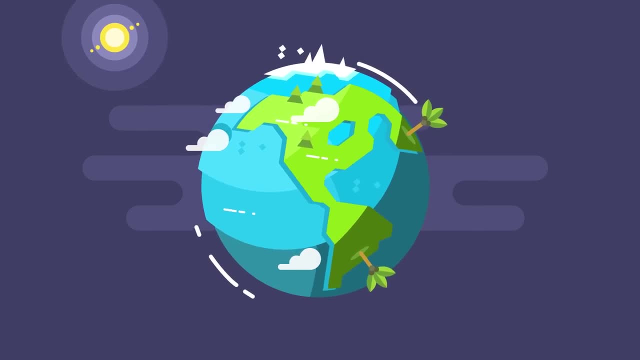 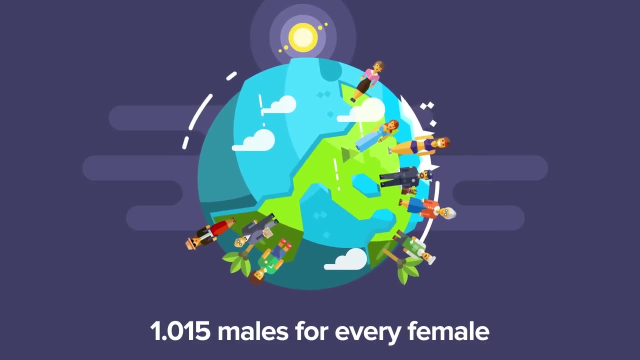 be part of our notification squad. In terms of sheer numbers, the men have the women of this world beat. In 2016,, the CIA of the United States estimated that there are approximately 1.015 males for every female. That may not seem like a lot, but with a world population of around 7.5 billion people, that's. 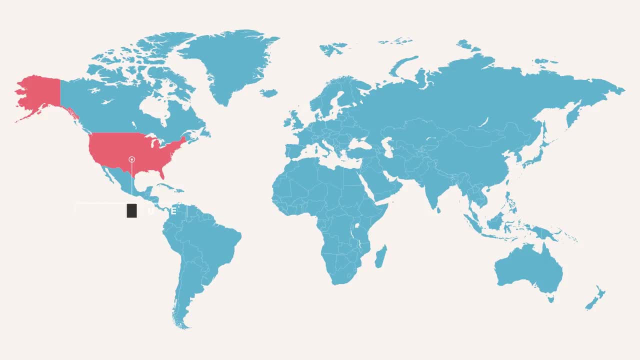 quite a few more guys playing for Team XY. According to data from the United Nations, the Great Cup of the United States is a little more full, with females having about 102 women for every 100 men. If you're looking for even more female friends, you might want to. 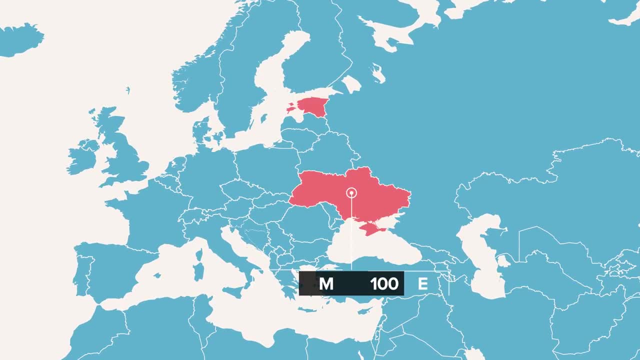 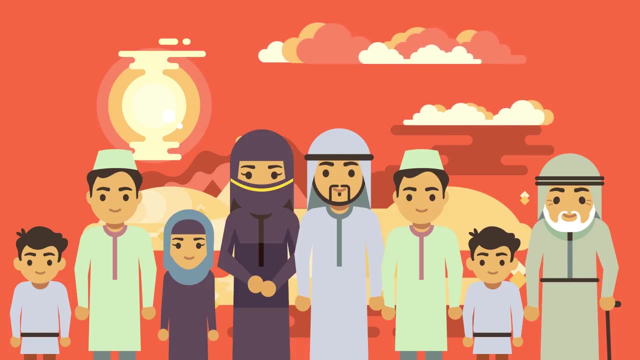 head over to Ukraine and Russia. Both places have the greatest relative amount of women in the world, with about 117 women for every 100 men. If you're on a quest for a greater concentration of Y chromosomes, Qatar might be just the place for you. It rings in at having the highest relative amount. 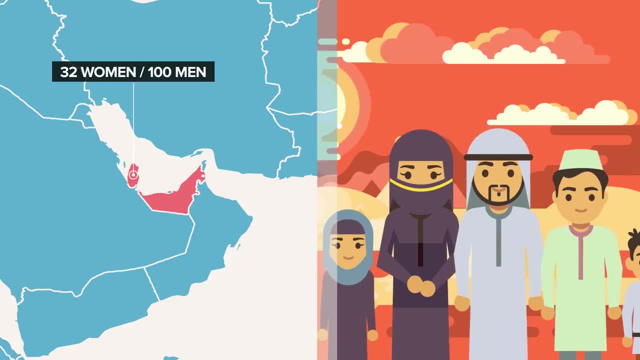 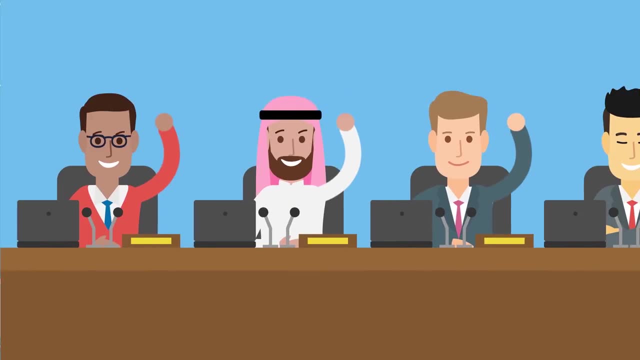 of delightful dudes, only having about 32 women for every 100 males. The United Arab Emirates is pretty similar, having 44 women for every 100 males, Even though there are almost as many women as men overall. the lovely ladies around the 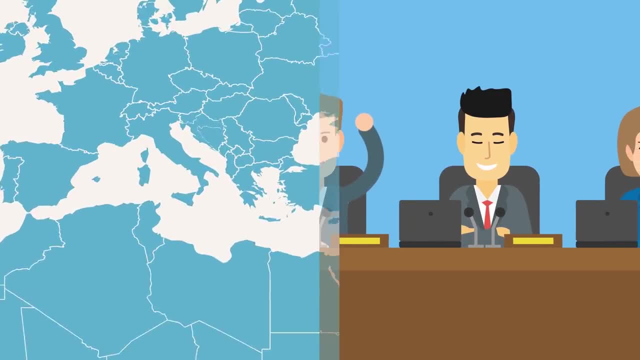 world only even beat the men of the United Arab Emirates. The United Arab Emirates is one of the few countries in the world where women can get an equal representation in parliament to men in the nation of Andorra, based off of 2012 data from the UN. Everywhere else. 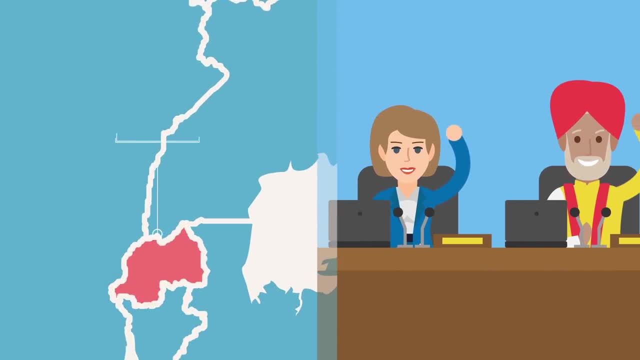 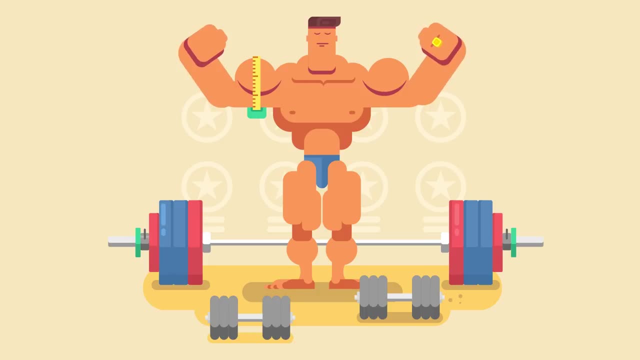 there are more parliamentary seats given to men than women other than in Rwanda, where women make up 56.3% of the parliament. When it comes to the battle of size, men are typically the heavyweights in the arena. According to the CDC, the average American male is 69.3 inches tall and weighs in at about 195.5 pounds. 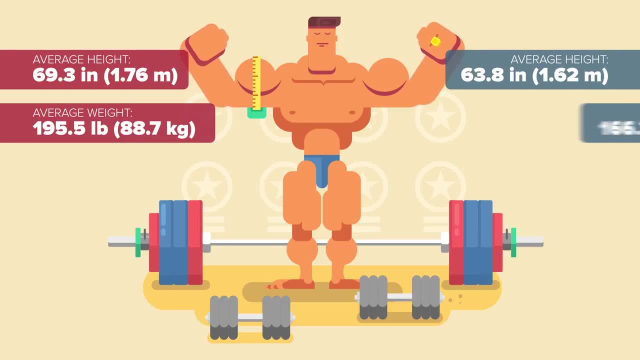 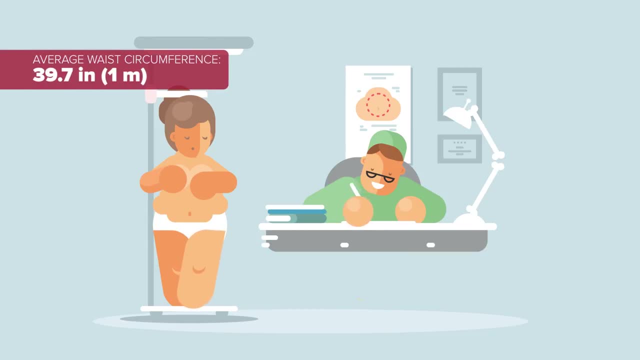 with the average female coming in at 63.8 inches and 165.5 pounds. Men are also a little thicker in the waist, with an average waist circumference of 39.7 inches, while women only measure about 37.5 inches in their waist circumference. If life 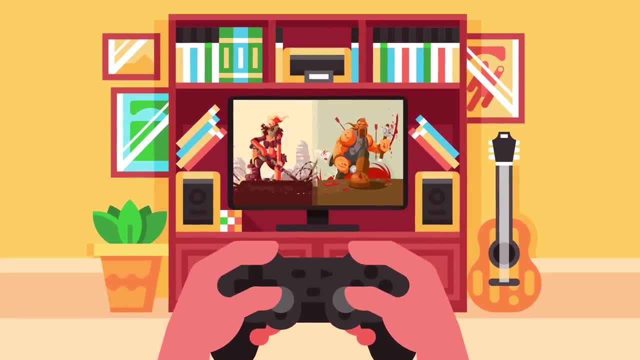 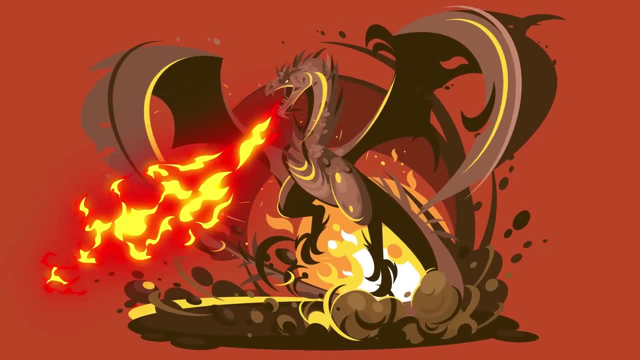 truly was an RPG. this could make women better suited for the light rogue class and men better suited for the heavy warrior class. Either way, I just want to slay some dragons and unlock treasure chests of gold. Women tend to live longer than their male counterparts, Based off of 2013 statistics. 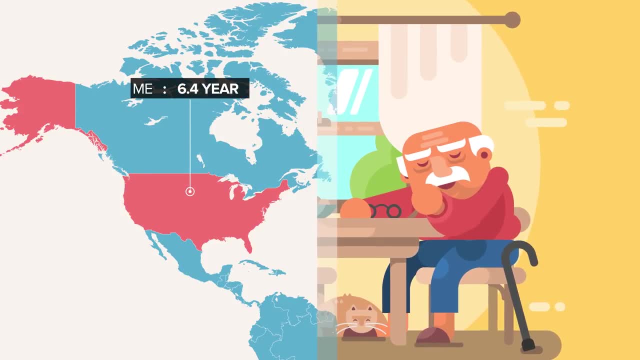 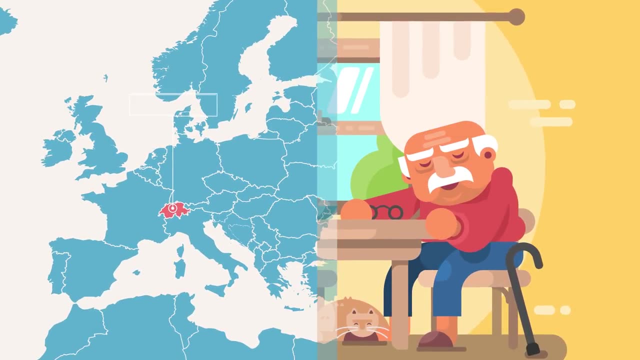 men in the United States had a life expectancy of about 1.5 million years. while men in the US had a life expectancy on average of 76.4 years, Women have an average life expectancy of about 81.2 years. With the reported countries, Switzerland had the longest life expectancy. for men at 80.7 years, and Japan had the longest life expectancy for women, at 86.6 years. One of the reasons for the gender differences in life expectancy can be traced back to rates of suicide and homicide between men and women. 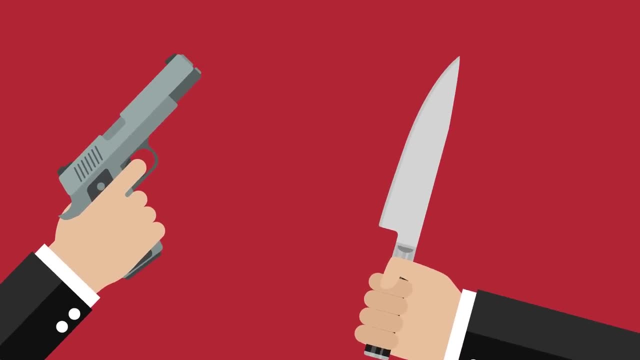 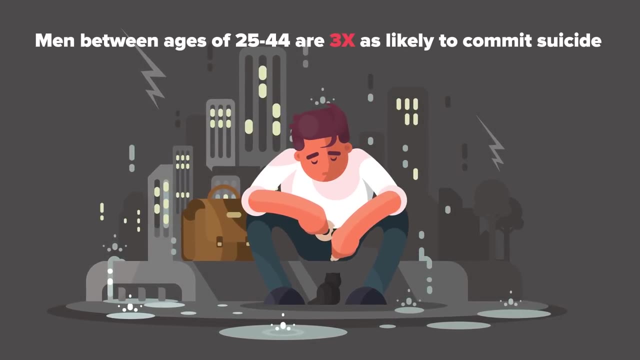 Based off of 2014 data, in the US, men had higher rates of both suicide and homicide than women. In the age bracket of 25 to 54, men were three times as likely to commit suicide than women, and the disparity was the greatest in the 65 and over bracket, where 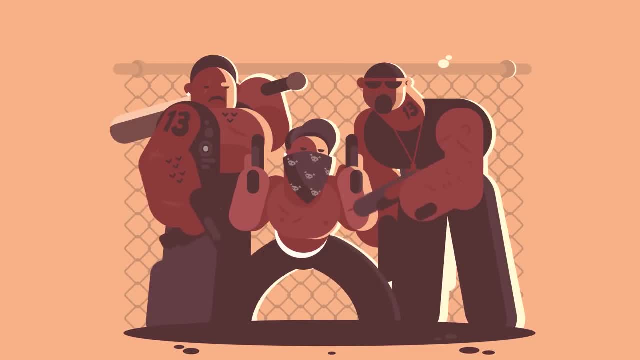 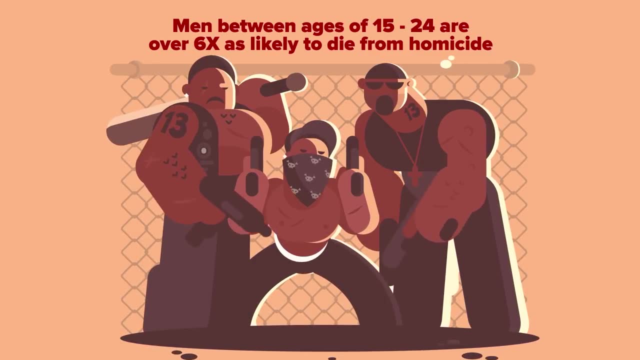 men were over six times as likely to take their own life Between 15 and 24 years of age. men were over six times as likely to die from homicide than women, but a little less than twice as likely for men to be a victim of homicide compared to women. when. 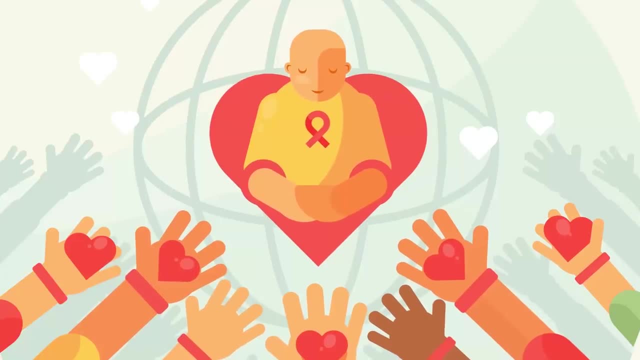 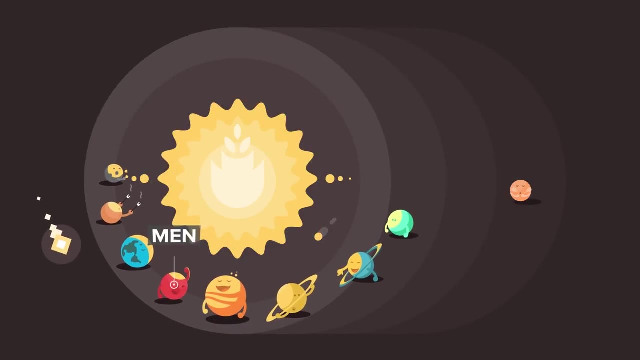 over the age of 65.. Both suicide and homicide can be devastating, and working to lower their rates among both sexes would be great fun. You may have heard the saying that men are from Mars and women are from Venus, driving a wedge between the sexes and making us think that men and women are significantly different. 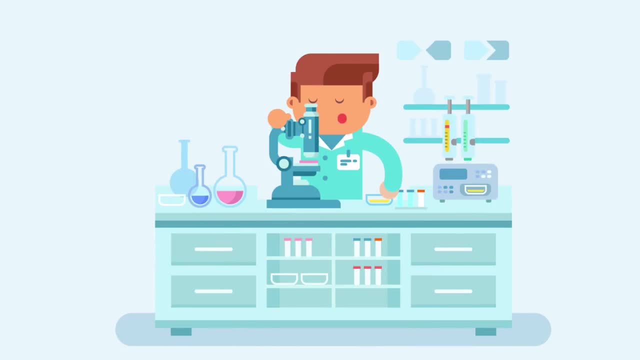 from one another. However, in reality, men and women seem to be far more alike than they are different. Based off the study of 46 meta-analyses, scientists found that men and women are basically alike in terms of personality, cognitive ability and leadership. Some differences were still. 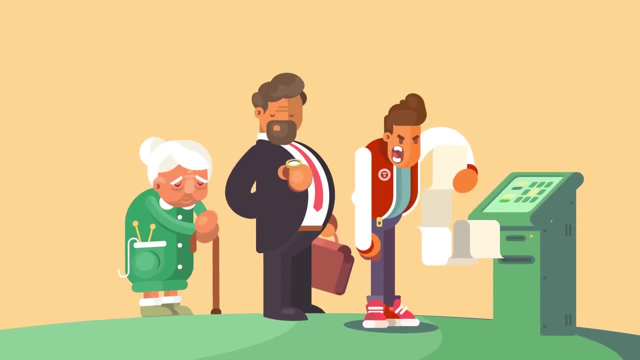 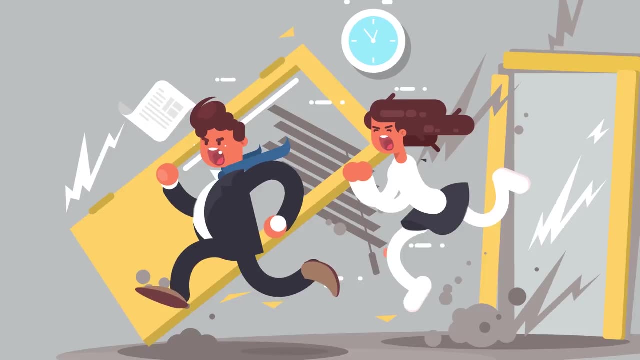 shown like men being slightly more aggressive, but even this seems to be more a product of society than men. In fact, in some studies designed to eliminate gender norms, women were more aggressive and men were more passive when the tests were designed to strip them of their stereotypes. 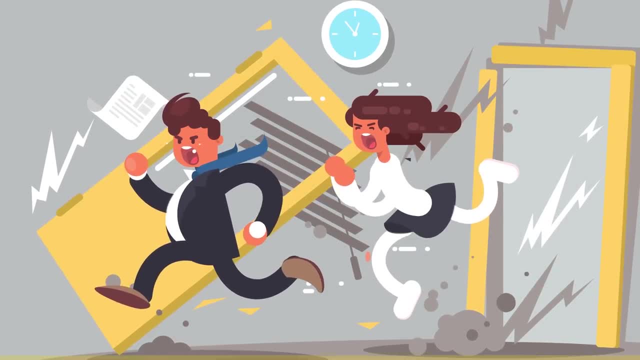 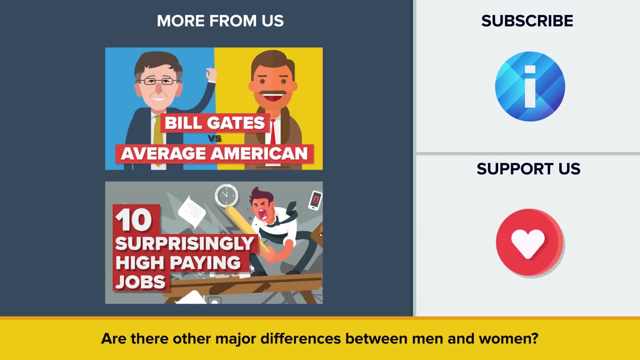 See, friends, don't let gender define you. Be whatever type of person you want to be. So are there other major differences between men and women that we failed to share in the video? Let us know in the comments. Also be sure to check out our other video called. 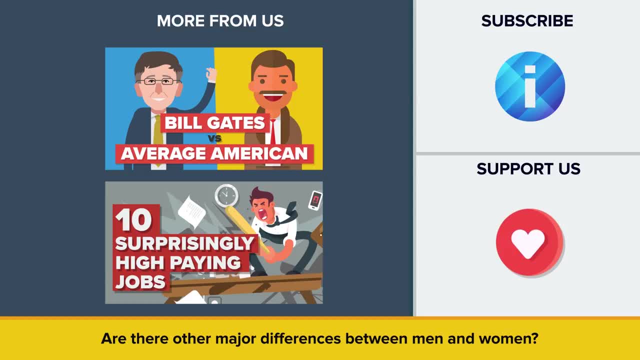 Bill Gates vs the Average American. Thanks for watching and, as always, don't forget to like, share and subscribe. See you next time. 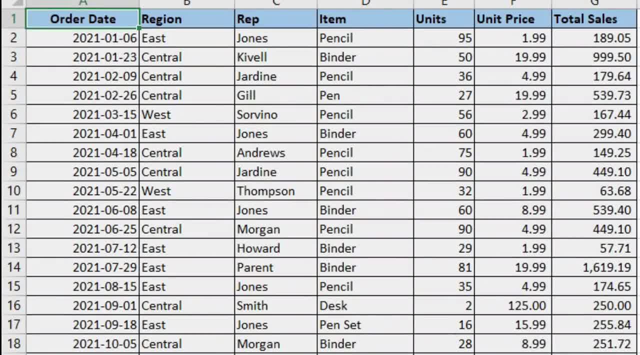 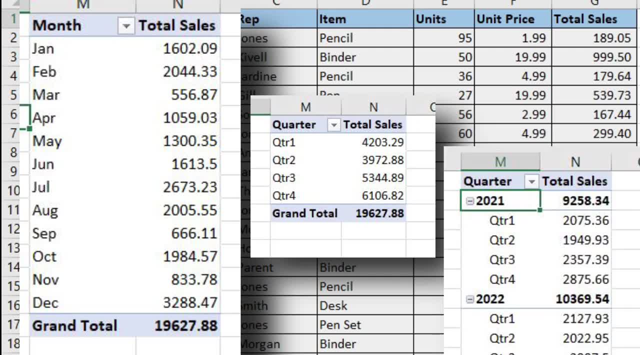 what if you have date wise sales figures, like i have here, and you want to calculate total sales for each month, or total sales for each quarter of the year or total sales for each year? with the help of pivot tables, you can get the desired data in just a few clicks.